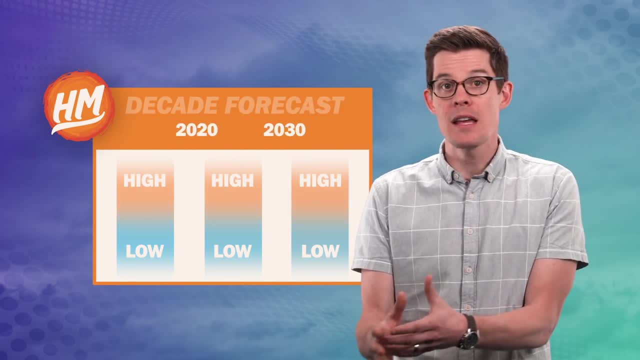 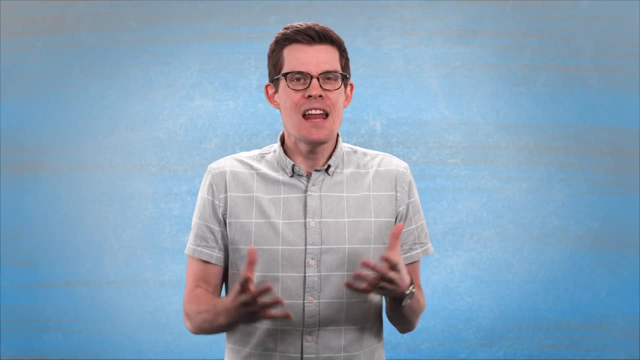 what you get if you take the weather over an entire year, decade or even century and look at it all together over a long timescale. But if they're so different, why does the day-to-day weather have such a strong influence on how we feel about the climate? and if we 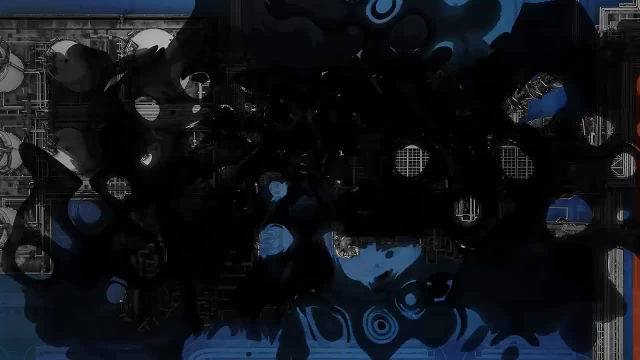 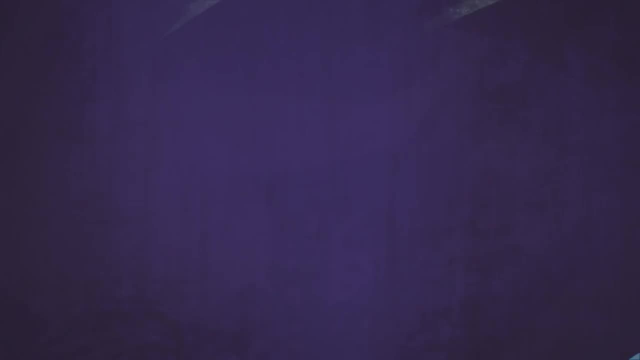 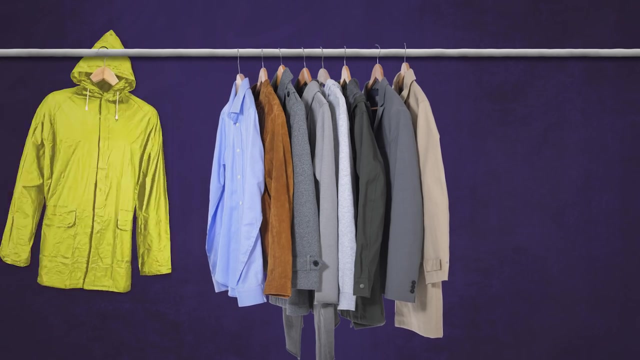 think the climate is changing. We can think of the day-to-day weather as the day-to-day weather, but it's also the difference between weather and climate. this way, Climate tells us what clothes to have in our closet and weather tells us what to wear right now. Sometimes we need a raincoat. 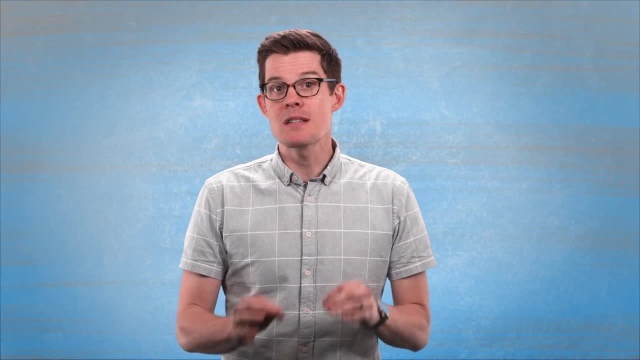 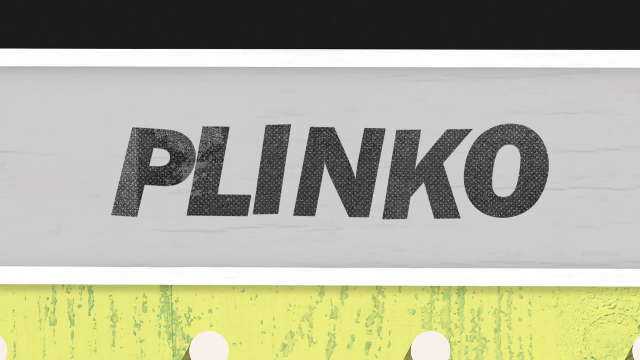 Other times we only need a t-shirt. That's because small disturbances in the atmosphere can lead to huge swings in the weather we experience every day. Ever seen that game Plinko? We don't know exactly where any one piece will land It. 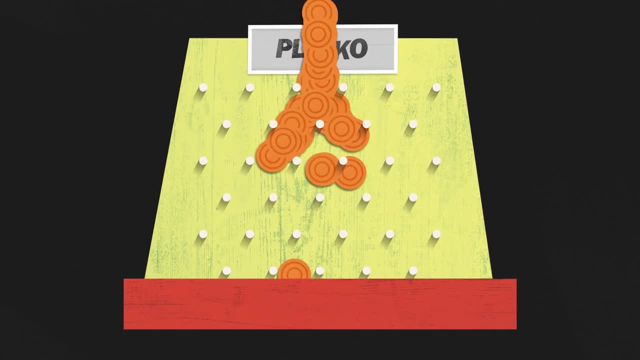 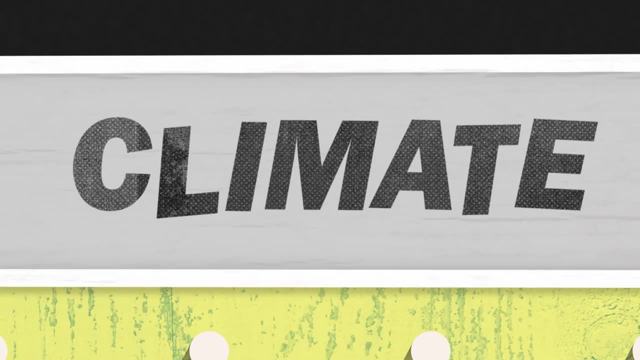 can go in a lot of different directions, But over many rounds a pattern will always emerge. Most pieces fall in the middle and fewer fall on the edges. Climate works the same way, Just like the Plinko pieces. we don't know exactly what. 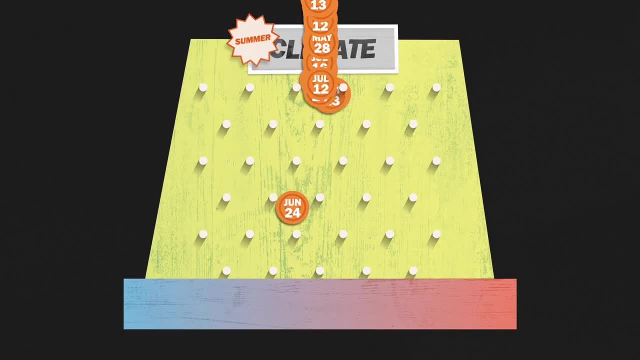 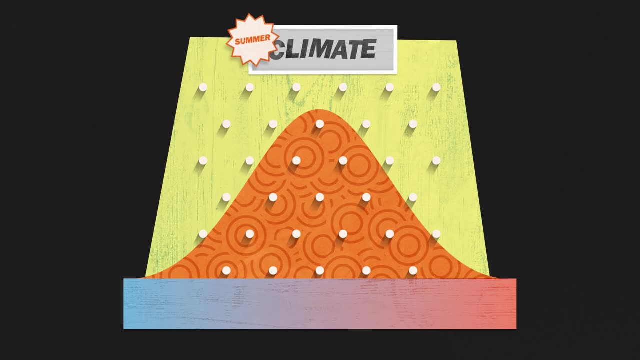 weather any particular day will have. But when we add up lots and lots of weather over many years, a pattern also emerges. This is the climate of any one place. It isn't very cold or very hot very often and most days are pretty normal for that place. 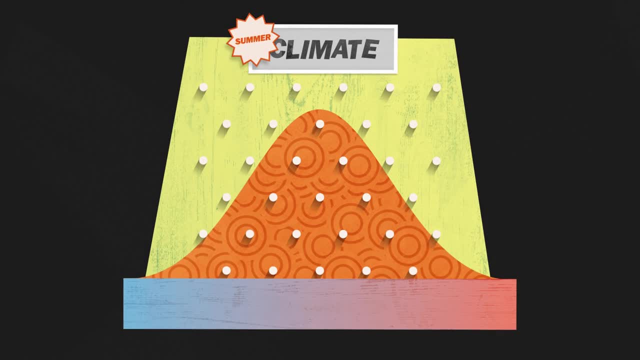 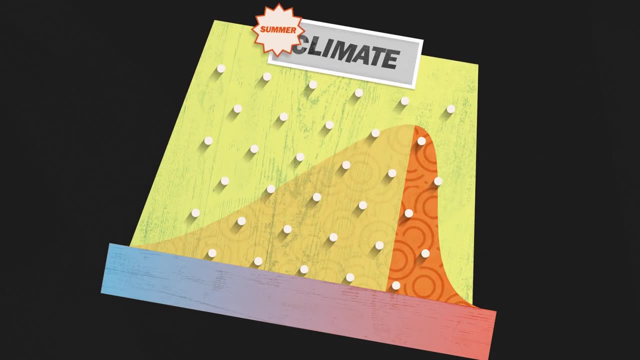 But when we look at the climate of any place over time, we can see that the pattern is changing, As if the Plinko board has been tilted. Most years have more hot days and fewer cold days than before, and the average day is getting warmer. 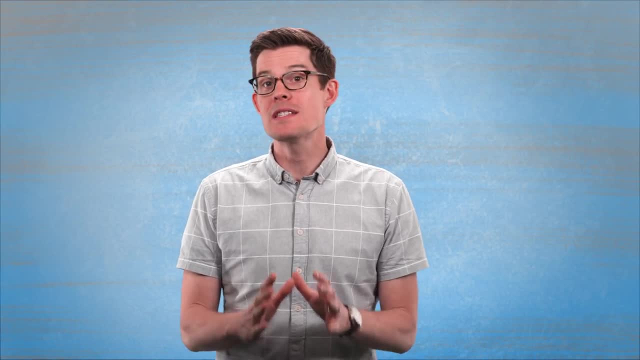 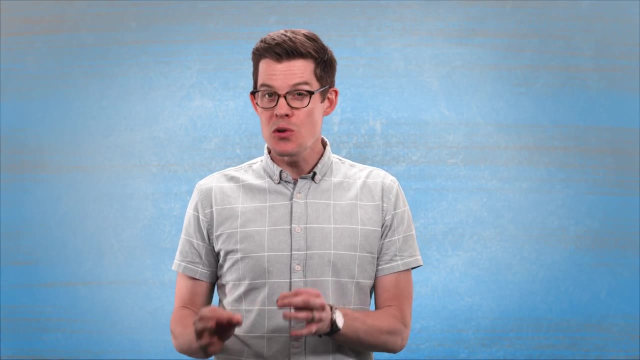 Day to day, we can't feel this shift in the climate, so instead we draw on our daily experience – weather – to explain what's happening. If we've recently experienced unusually warm weather, we're more likely to believe the climate is warming and more likely to be concerned about the consequences On the 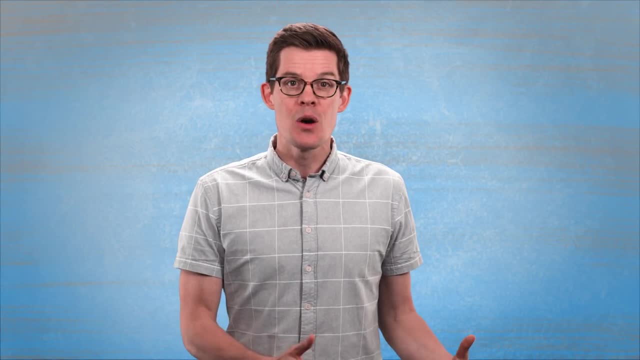 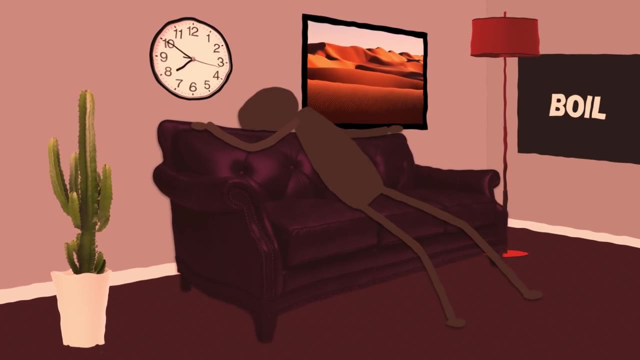 other hand, if we've experienced a lot of unfavorable weather, we're more likely to feel the climate warming. experienced a lot of cold days, we're less likely to believe the climate is changing. In one study, participants who either sat in a warm room or read words that sound hot. 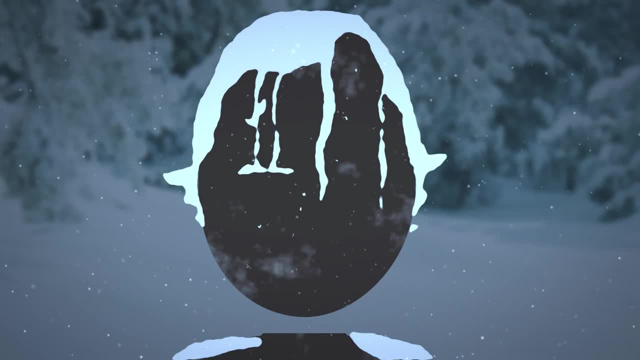 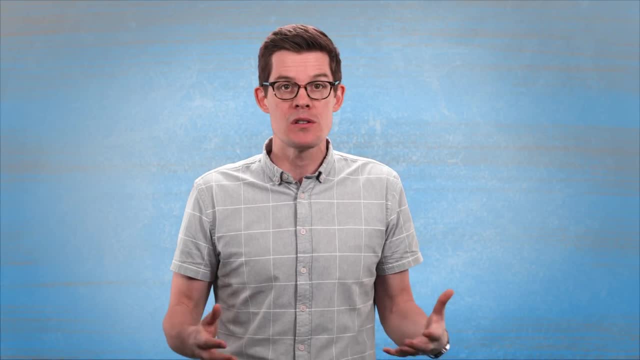 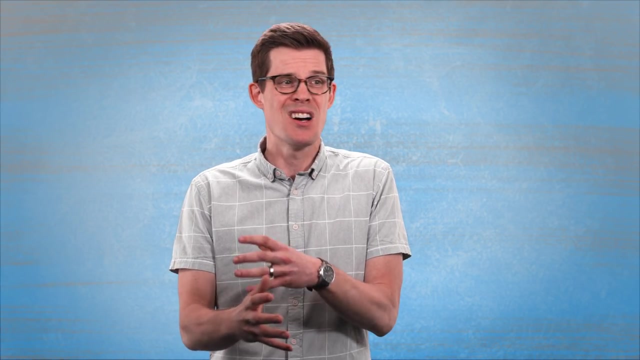 were more likely to believe that the climate is changing than participants who sat in a cooler room or just read neutral words. This happened because our brains tend to make judgments using whatever information is most readily available. This mental shortcut allows our recent memories and experiences to fool us on all kinds of 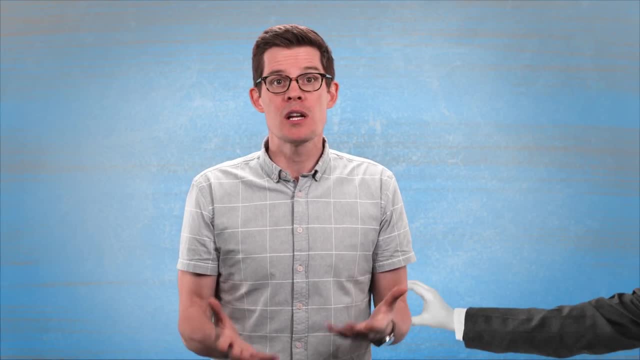 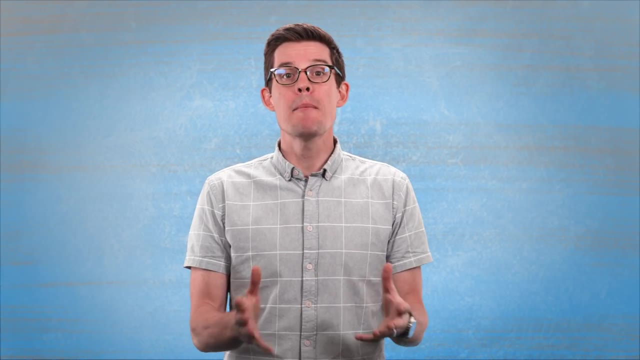 issues, Our views on crime. they'll probably be different if we've just been robbed. Our views on the economy depends on if we just lost a job. When we're faced with a complex, difficult issue like climate change, instead of carefully 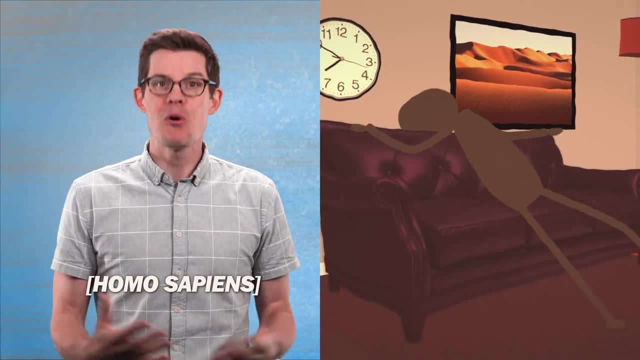 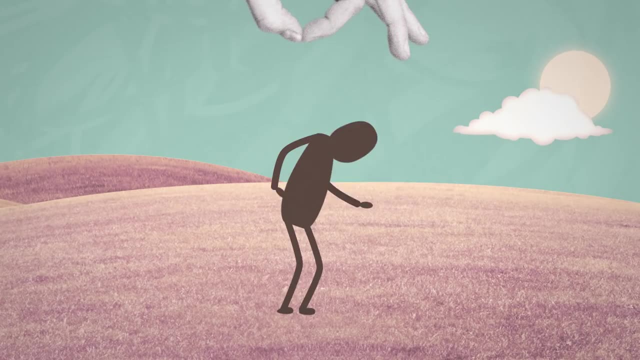 analyzing it, like the rational beings we think we are. we base our judgment on more recent experiences that relate to it, like the weather. So, because we experience the weather, it's often at the front of our minds and we talk about it. 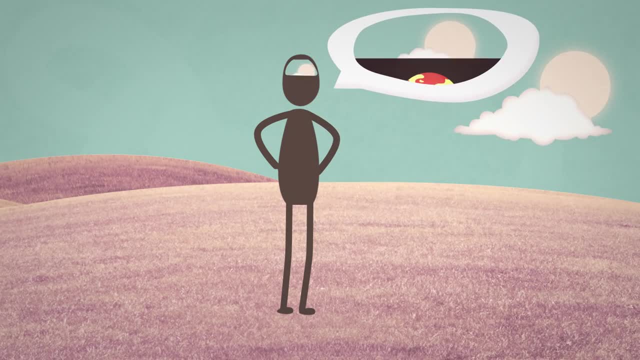 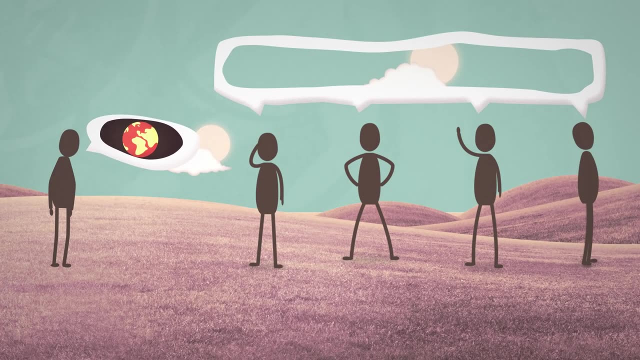 And because we talk about it, it's more likely to stay there. But this doesn't happen with climate. In America, just one out of every five people has talked about global warming in the last month. Even among people who think global warming is important, less than half of them regularly. 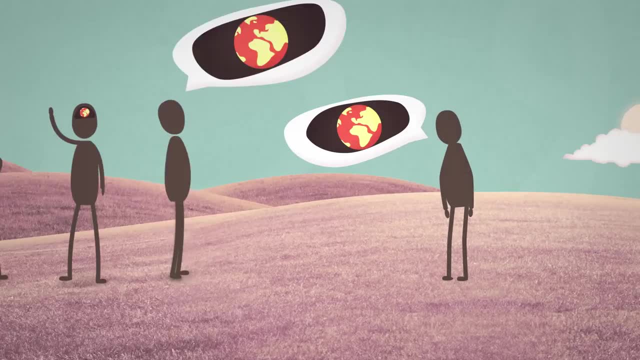 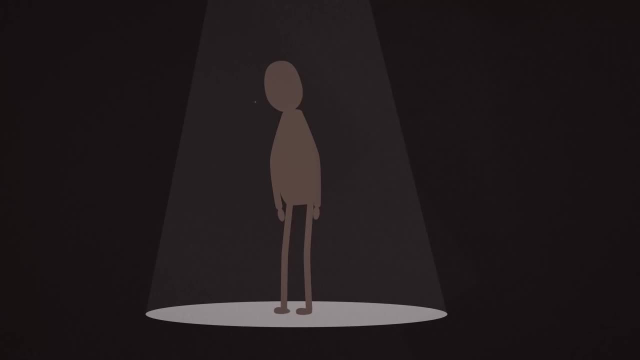 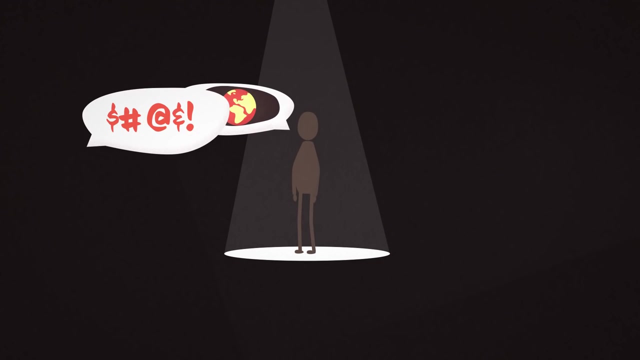 discuss it. Climate science More like climate silence. Even though most of us are concerned about climate change, researchers have found that we underestimate how many other people are concerned, So we often avoid discussing climate change because we assume most of the people around us will be concerned. 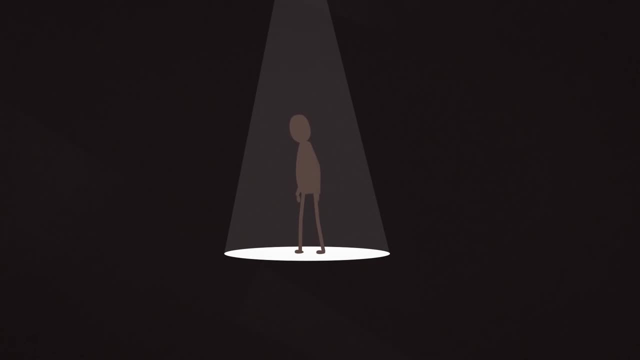 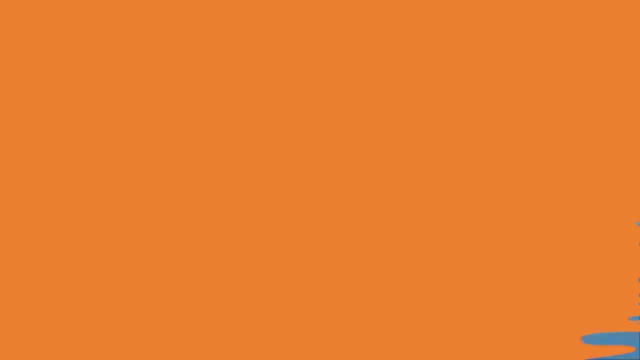 They'll disagree with us. But if we stay silent, it leads other people to believe their concern is uncommon, So they stay silent too. It's a spiral of silence, But just like the weather we all experience, the climate. It simply changes more slowly. 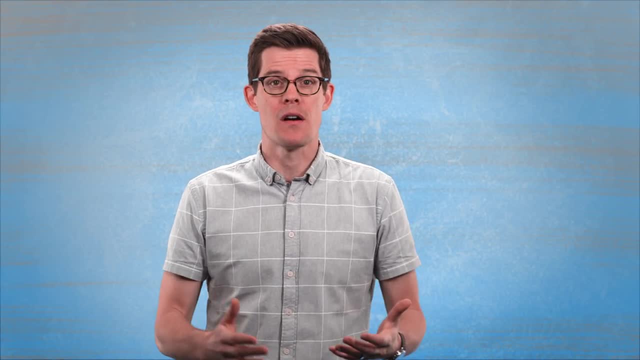 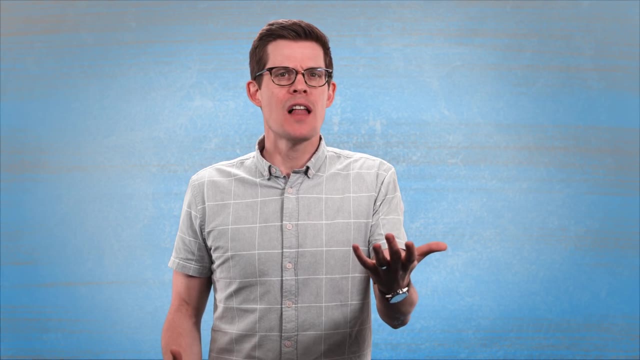 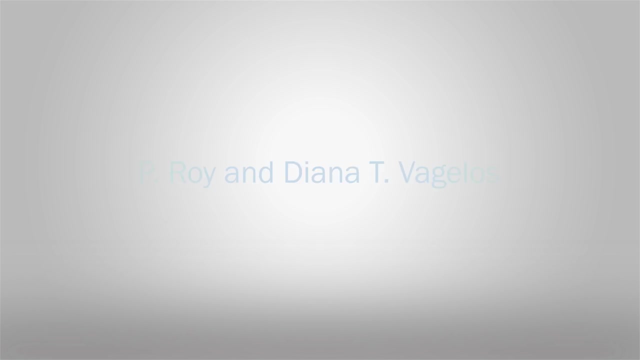 The effects of that changing climate are even more universal than the weather, So maybe we don't realize how many other people are out there waiting for us to ask: how's the climate these days? Fun to get to know. Thanks for watching. The funding for this episode is provided by these funders, P Roy and Diana T Vagelos. 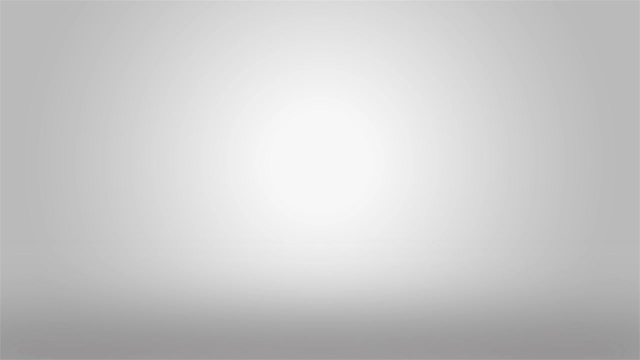 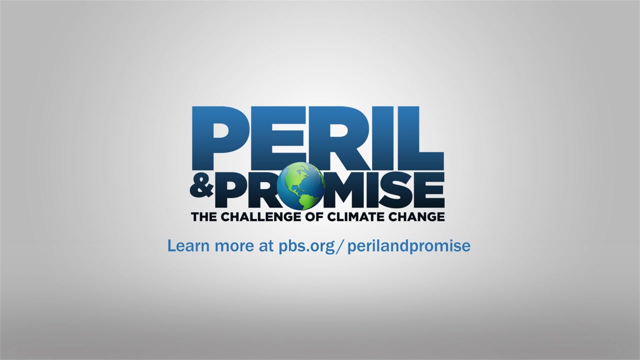 the Mark Haas Foundation and Sue and Edgar Wachenheim III in support of Peril and Promise, a public media initiative from WNET in New York reporting on the stories of climate change and its solutions. Learn more at PBSorg: slash perilandpromise.